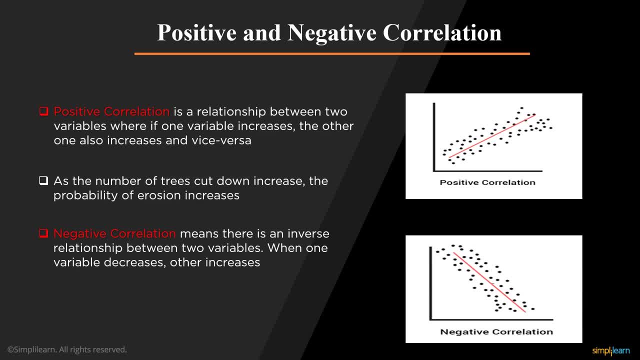 that the correlation is just the opposite. The relationship line has a negative slope, as you can see from the graph, and the variables changes in the opposite direction. That is, one variable decreases while the other increases. To understand this, an example can be if: 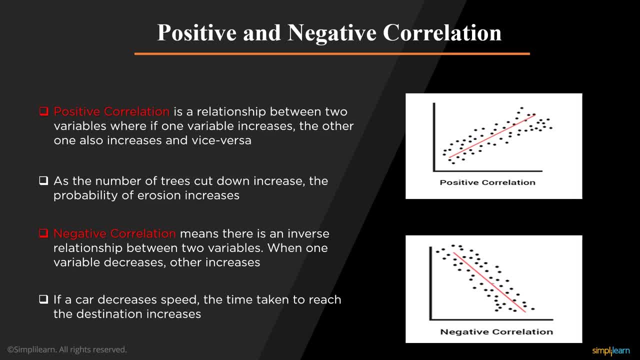 a car decreases the speed, the time taken to reach the destination increases. To know more about the types of correlation, you can refer to our previous videos and you can find the link in our description. What is regression? Regression analysis, like most multivariate. 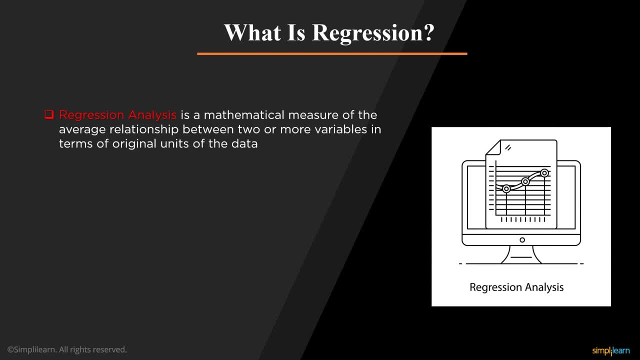 statistics allows you to infer that there is a relationship between two or more variables. These relationships are seldom exact because there is a variation caused by many variables, not just the variables being studied In regression analysis. there are two types of variable: One is dependent variable and other is independent variable. Let's discuss what the both variables. 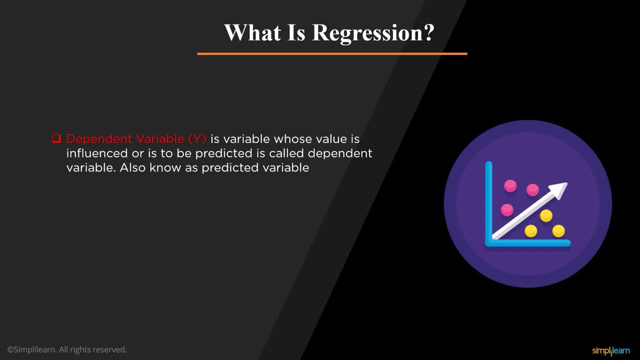 represent. A dependent variable is a variable whose value is influenced or to be predicted. The dependent variable is often denoted by y and is also known as the correlation variable. as you can see from the graph that I just told you, The dependent variable is a variable whose 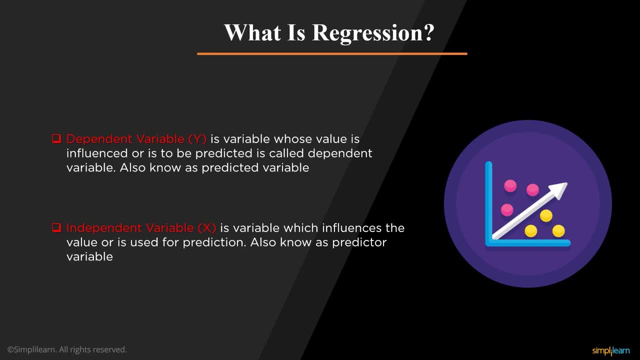 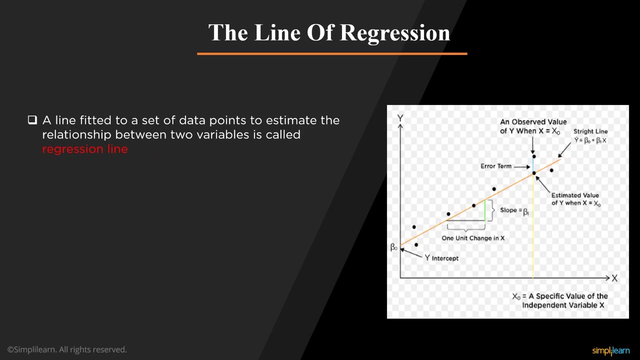 predicted variable, Whereas independent variable, which is denoted by x, is a variable which influences the value or is used for prediction. The independent variable is also known as a predictive variable, The Line of Regression. The regression line is a line which is used to describe the behavior of a set of data. 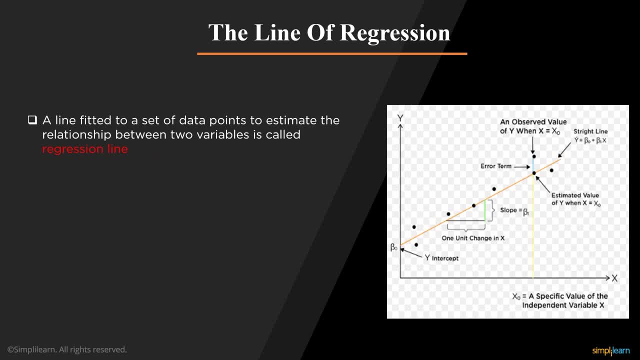 In other words, it gives the best trend of the given data. Regression lines are useful in forecasting procedures. Its purpose is to describe the interrelationship between the dependent variable and independent variable. The regression equation of y on x describes the change in the value of y for given changes. 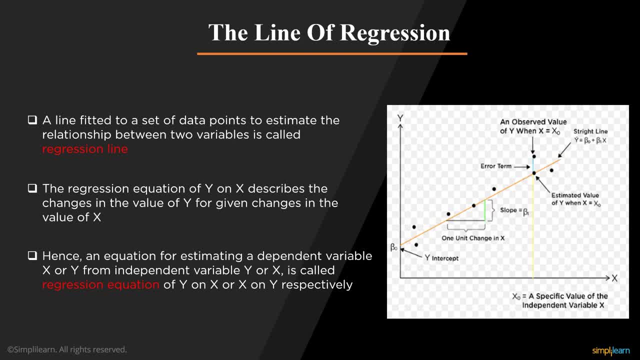 in the value of x and vice versa In the regression line equation. x and y are the variables of interest in our data, with y the unknown or dependent variable and x the known or the independent variable. Let's discuss the two key terms in this graph. The first one is slope. Slope is the ratio. 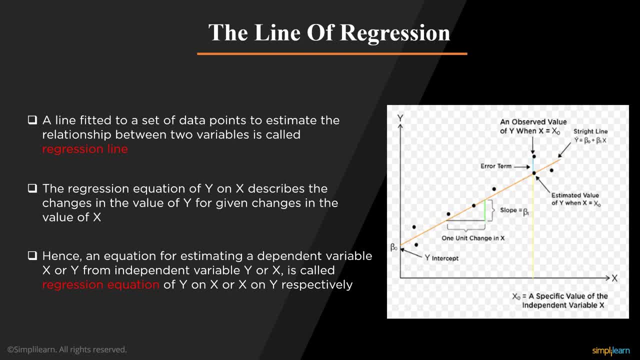 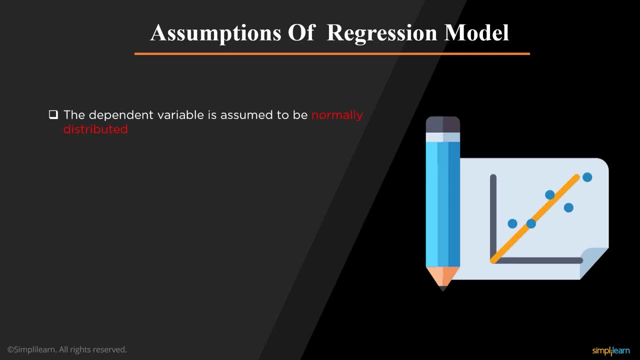 of the vertical and horizontal distances between the two points of the graph And you can see y-intercept, which is the coordinate of the point at which the curve intersects an axis. There are some assumptions we take to create the regression model. The first one is the 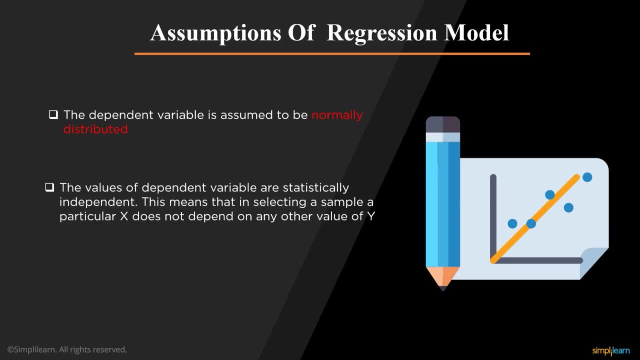 dependent variable is assumed to be normally distributed. The values of the dependent variable are statistically independent. This means that when we select the sample of a particular x, it does not depend on any other value of y. And the third one is error. values are statistically. 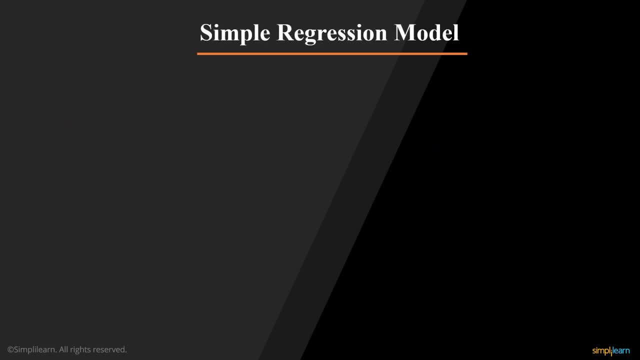 independent. Now let's discuss a simple regression model. A simple regression model is used to depict a relationship between variables which are proportional to each other, Meaning the dependent variable increases, decreases with the independent variable. The equation of a simple regression model is: y is equal to b0 plus b1x plus e, Where 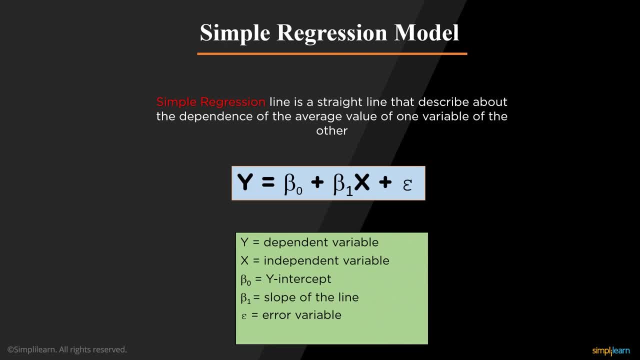 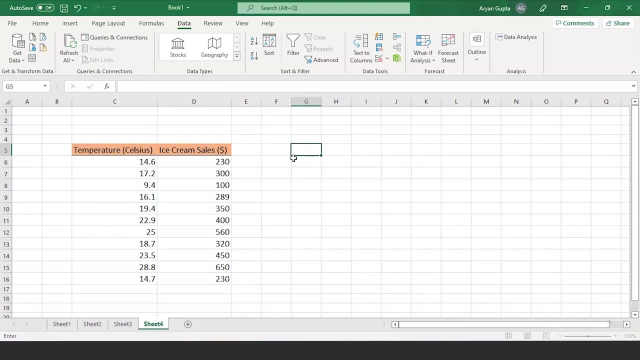 y is dependent variable, x is independent variable. b0 and b1 represents y-intercept and the slope of the line respectively, and e is the error variable. Now let's move on to excel to calculate the regression coefficient. We are on an excel workbook. In front of us we have the data of temperature of the day. 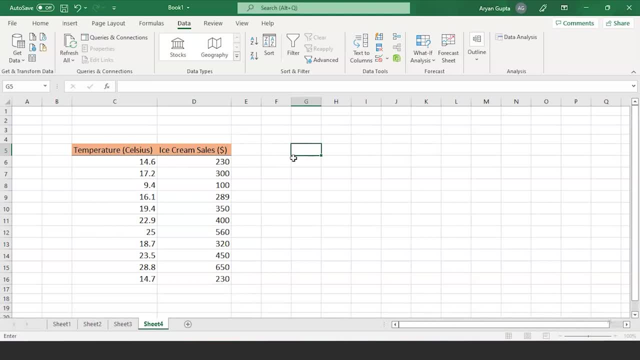 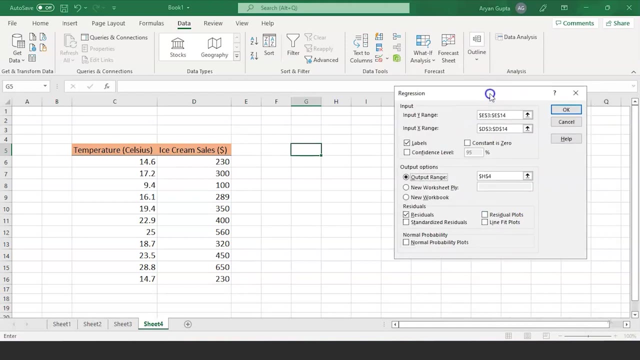 and sales of the ice cream on that day. Let's try to understand its regression, analysis and summary output using this data. So the first step is to go to the data tab and select data analysis, Then select regression and click ok. We will get this table. Select the y range as the ice cream sales. 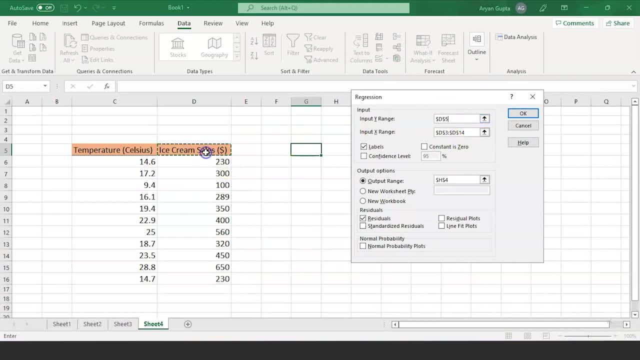 This y range is predictable variable, also called as dependent variable. For the input x range, we will select the temperature in degree Celsius. This is the explanatory variable, also called as the independent variable. One thing you should keep in mind is that both the x and y column must be adjacent to. 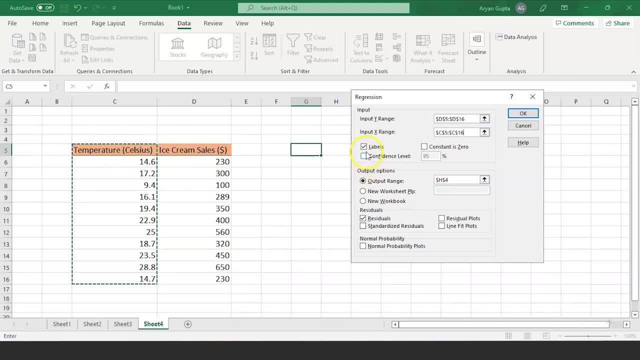 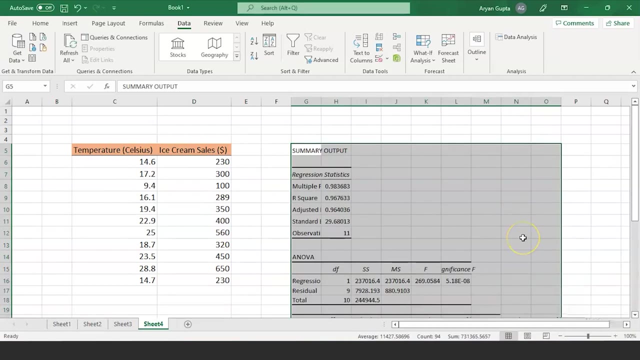 each other. We have the label, so we will check the label and we will select the output range from G5.. Check the residuals and click ok. Excel produces the following output: Let's analyze some key data. Let's analyze some key data. 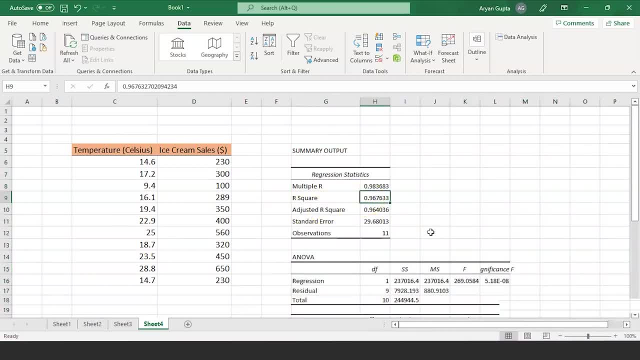